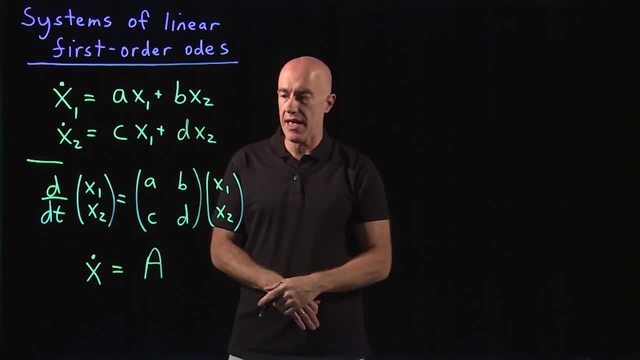 to a 2 by 2 matrix which I'll write capital A times the column vector x. So the system of first order linear equations can be simply written as: x dot equals A. So we've got a 2 by 2 matrix which is A times x. To solve this we're going to use an ansatz and we're. 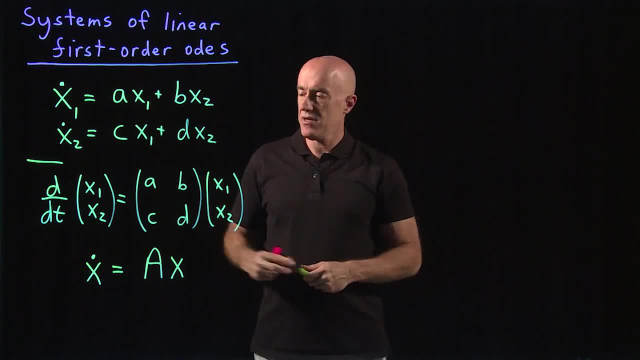 also going to use the principle of superposition. So we're going to look for solutions following our ansatz and then, when we find solutions- two solutions in this case- we'll multiply them by constants and add them together to get the general solution. So what is the right? 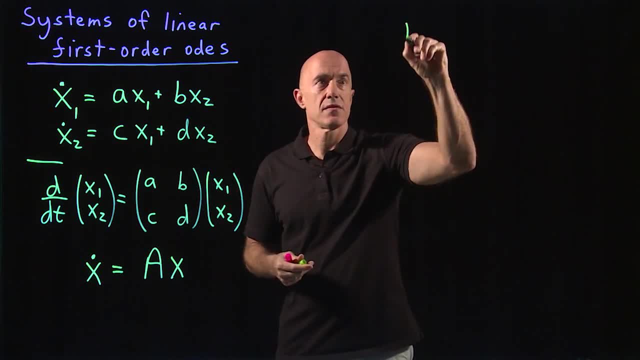 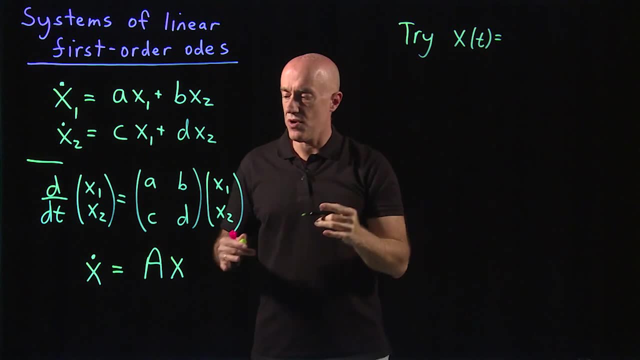 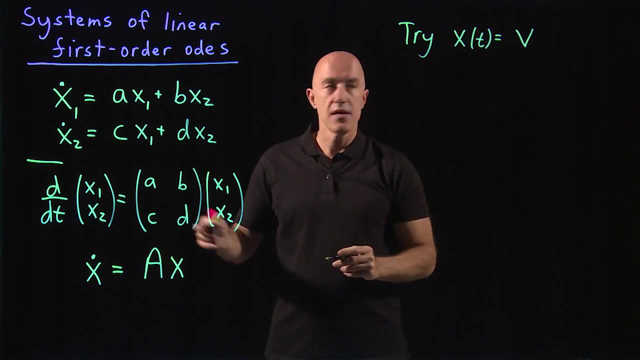 write onsatz here. we're going to try x of t, the column vector equal to a constant column vector, which I'll call v. so this is a 2 by 1 matrix times an exponential, and we'll call that e to the lambda t. okay, That will be our onsatz, And then we're looking. 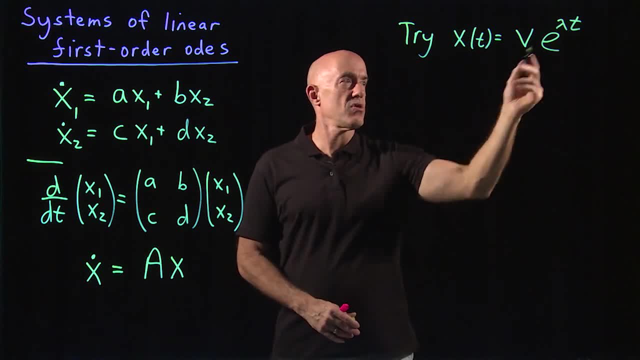 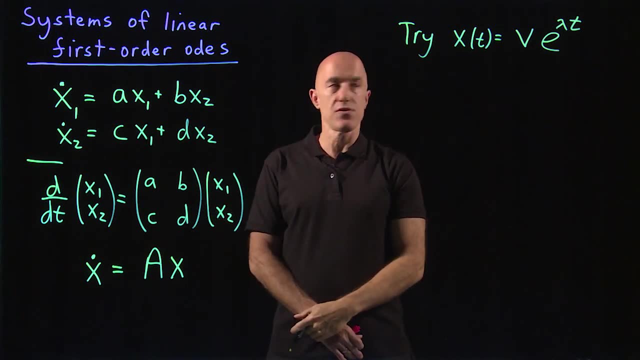 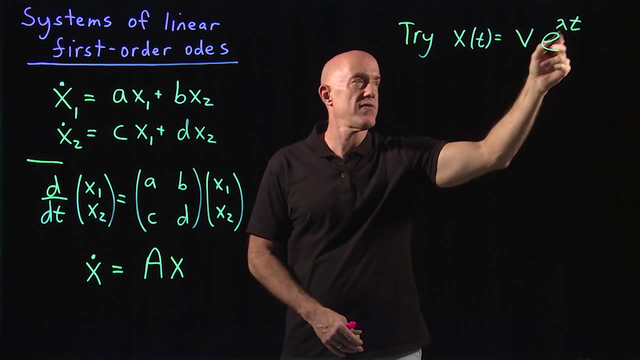 for here, in this type of onsatz, we're looking to determine both lambda and v. What happens when we substitute into the differential equation The time derivative? v is independent of time. the time derivative will bring down a lambda. lambda is also independent. 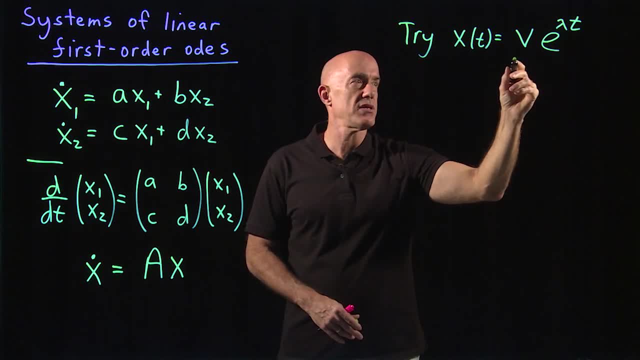 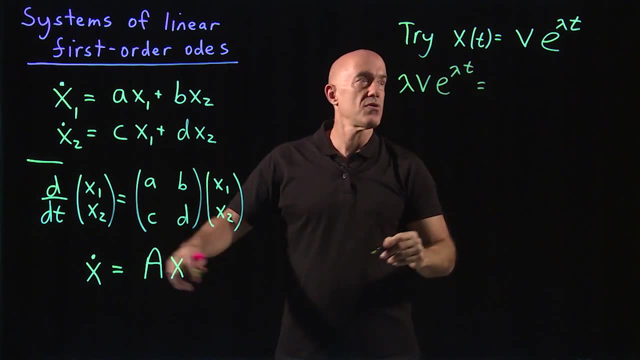 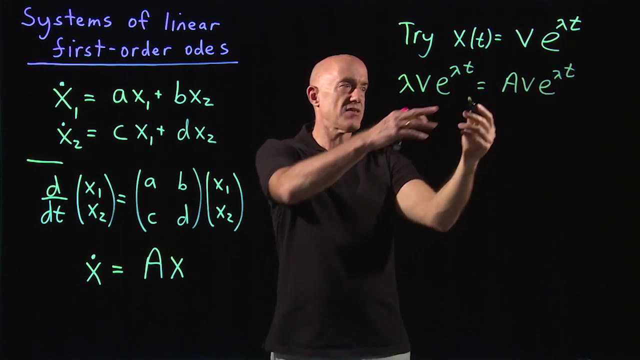 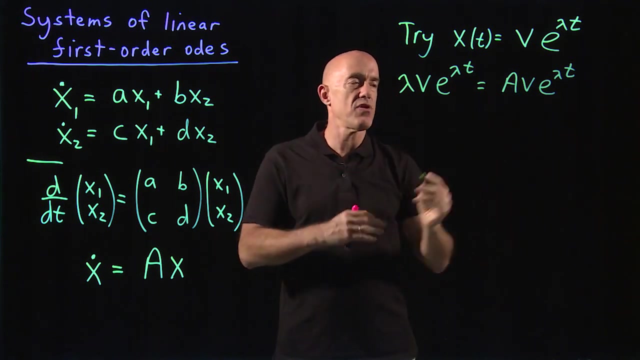 of time. so substituting into the differential equation, we'll get: lambda v. times e to the lambda t Is equal to a times v times e to the lambda t, As always the exponential cancels. that's the point of the exponential onsatz. and rewrite this in a more telling fashion: put the av. 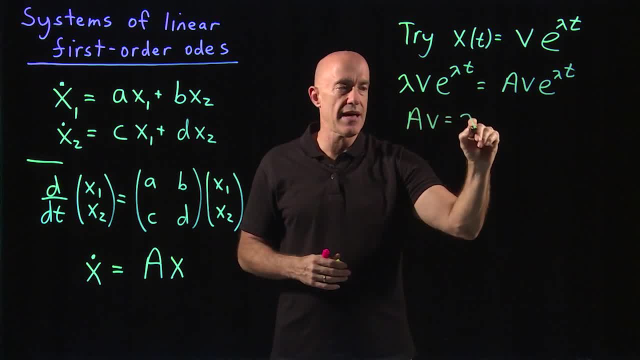 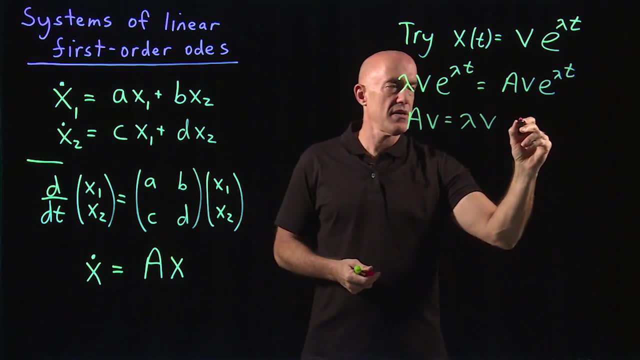 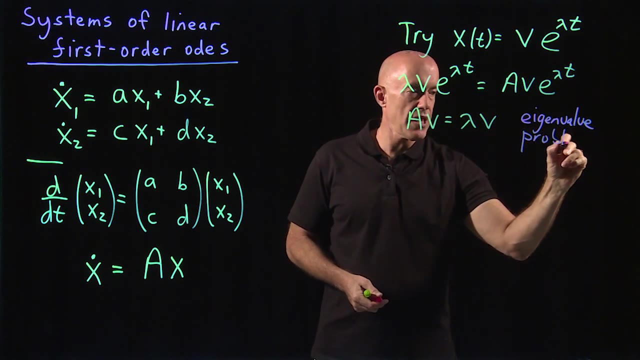 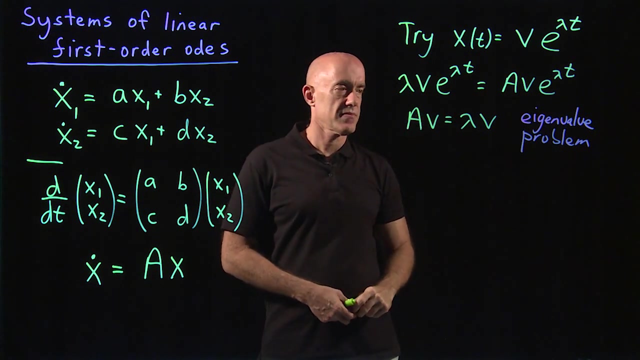 on the left, we get av equals lambda v. Those of you who remember your matrix algebra, this is the answer. This is the eigenvalue problem. So lambda are the eigenvalues of the matrix A and v are the eigenvectors. How do you compute the eigenvalues? You use the characteristic. 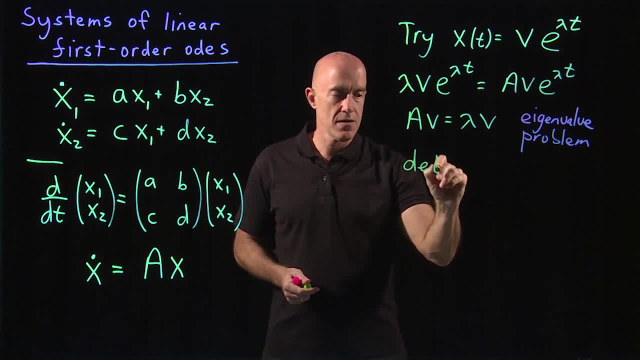 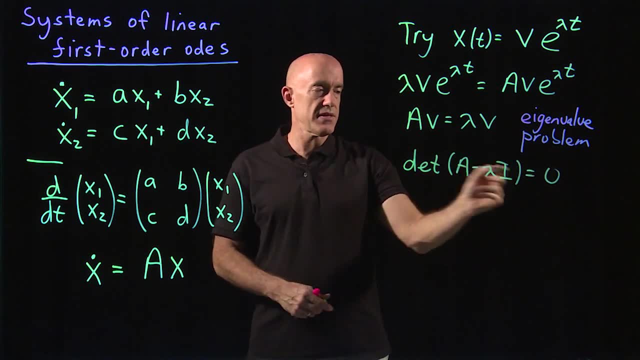 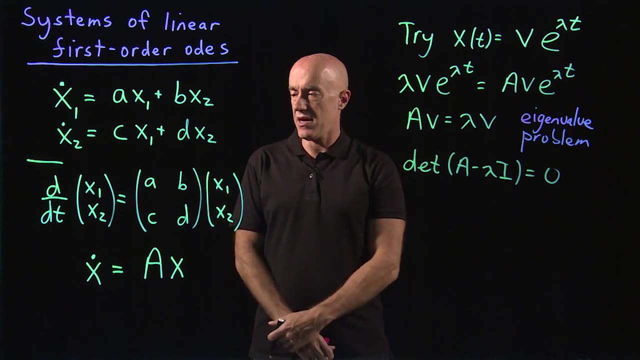 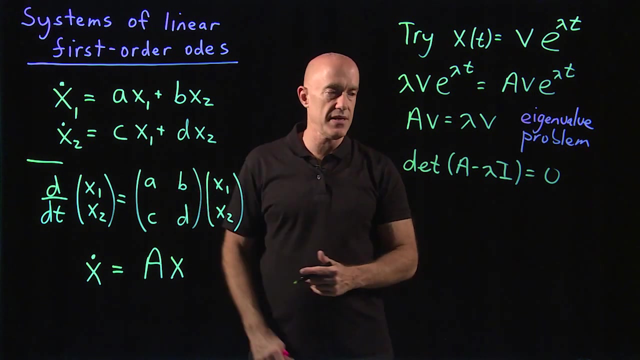 equation which is the determinant of A minus lambda I equals zero. This is a quadratic equation for lambda, If you remember your determinant of the two by two matrix: the A minus lambda on the diagonals, and b and c off, this equation becomes lambda squared. 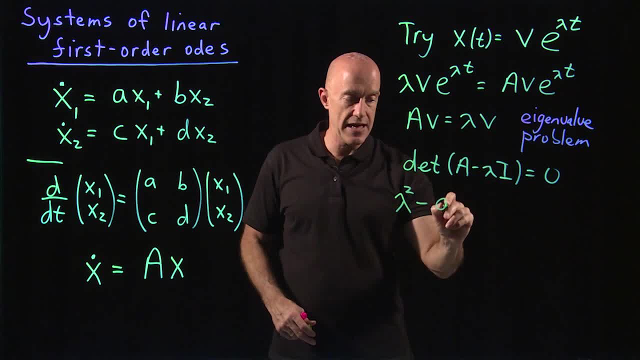 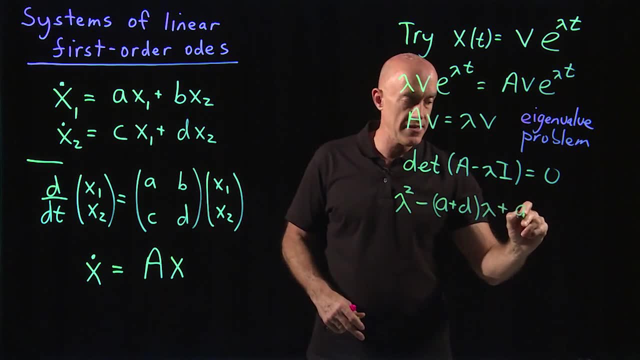 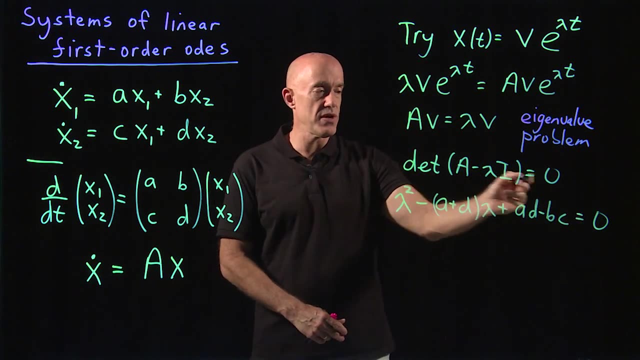 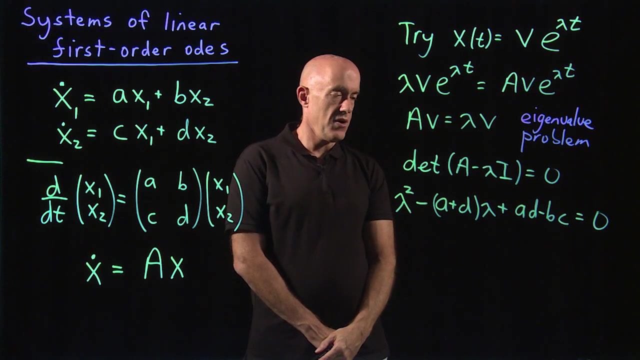 minus the trace of the matrix A, plus d times lambda, plus the determinant of the matrix A d minus b c, So you get a matrix A equals zero. That's doing this determinant and if you remember this from a matrix algebra course, 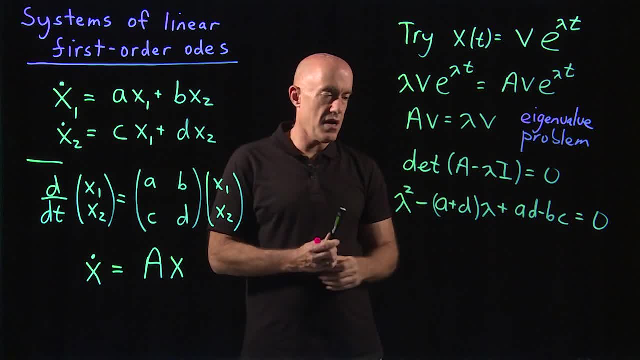 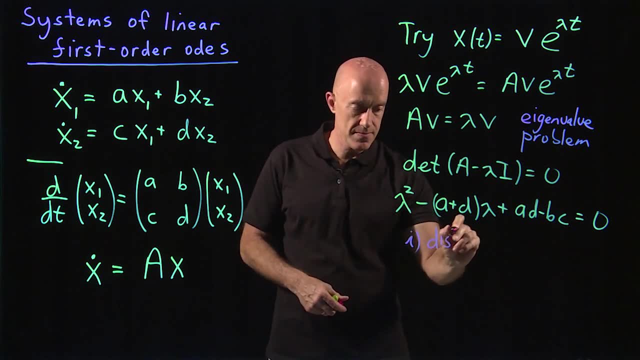 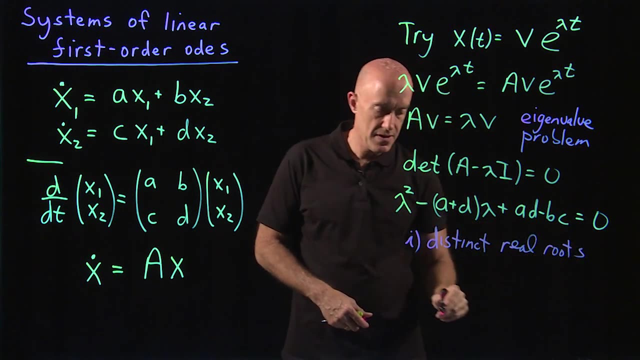 Three things can happen in a quadratic equation. What are they? The first one is that you can have distinct real roots for the eigenvalue lambda. The second one is that you can have distinct real roots for the eigenvalue lambda. The second thing that can happen is you can 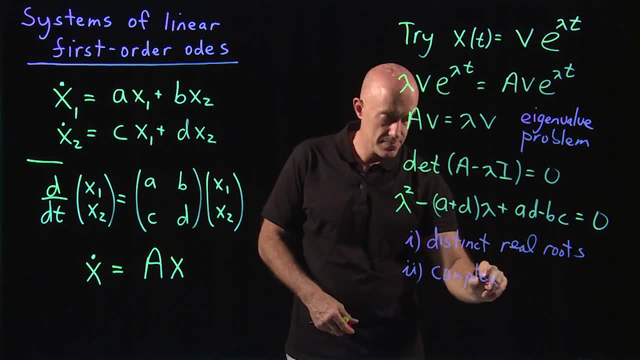 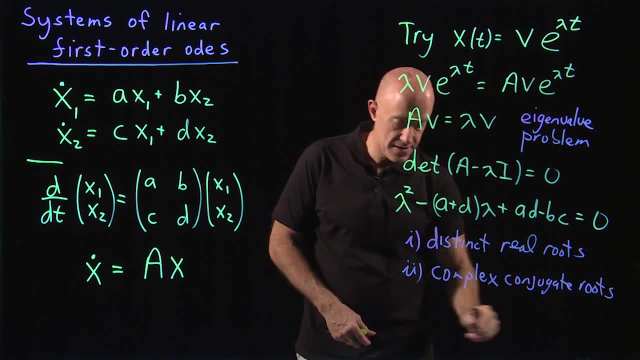 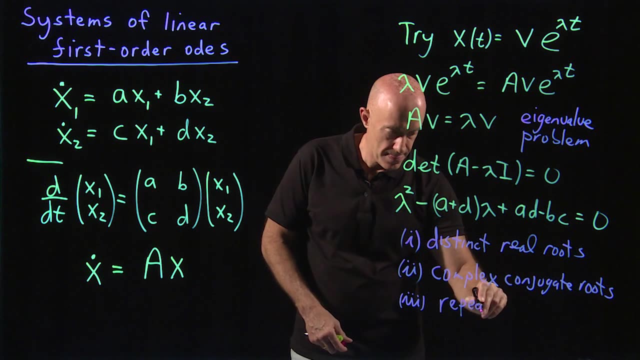 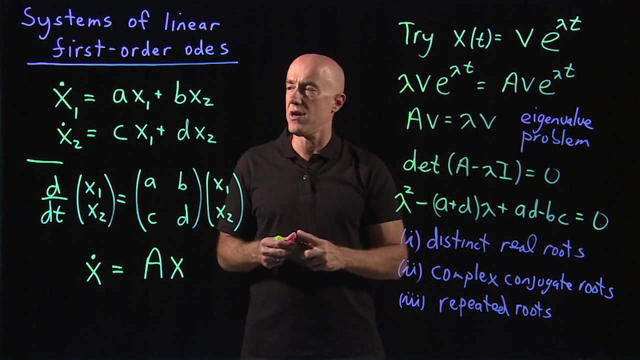 have complex conjugate roots And the last thing that can happen is you can have repeated roots. Okay, Sound should be sound very familiar to the second order: linear derivative equation, homogeneous equation with constant coefficients, because actually it's the same thing. okay, but look that in a different way. in this course we'll 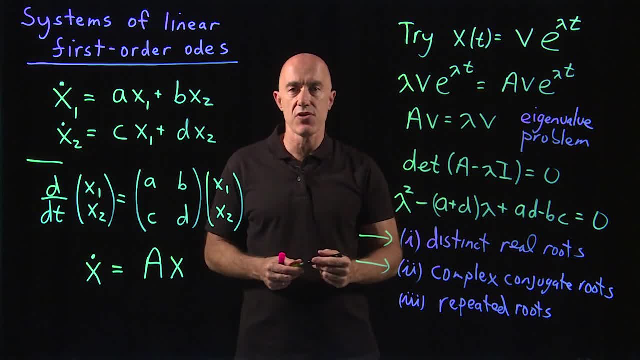 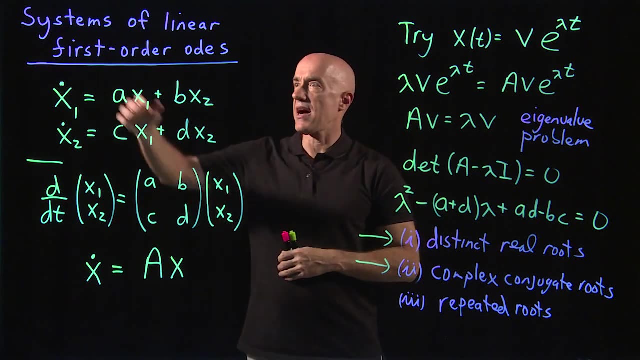 consider these first two cases and we'll skip this third case, which is a bit too specialized for the time that we have to learn differential equations. okay, so let me summarize. we're now considering how to solve a system of linear first order equations. for simplicity, we'll consider two equations: an equation for x1 and an.